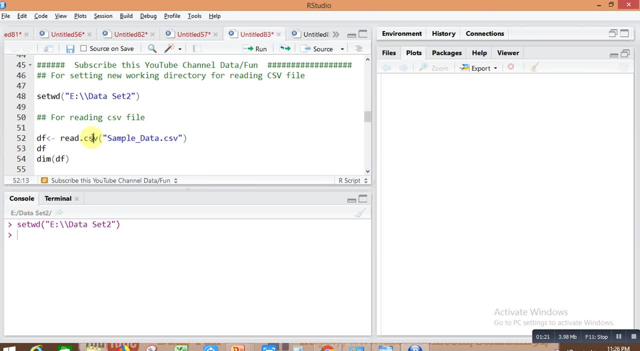 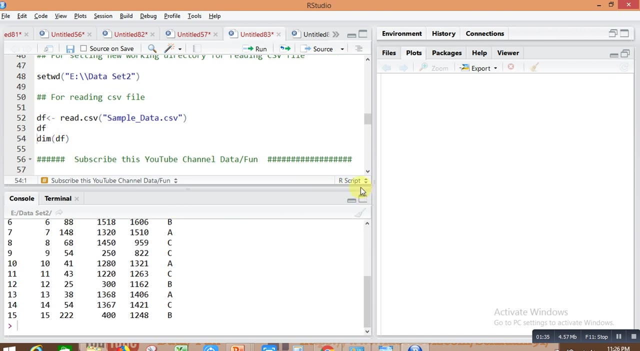 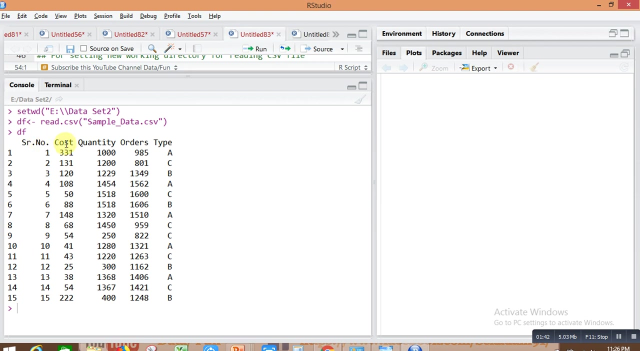 format of csv. that's why i am use readcsv command for reading sample underscore dot csv file and i am giving the data frame name df. let's see what is the data. so first column of data is serial number, second is cost, third is quantity, fourth is order and last one is: 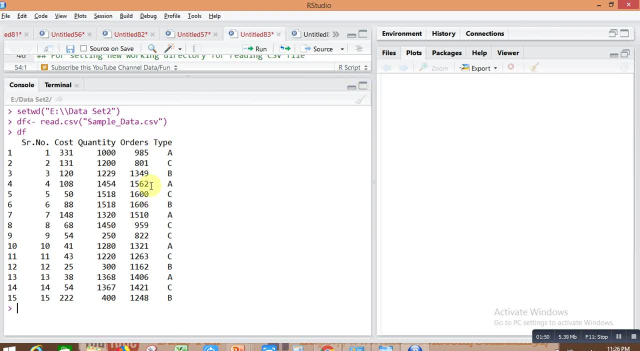 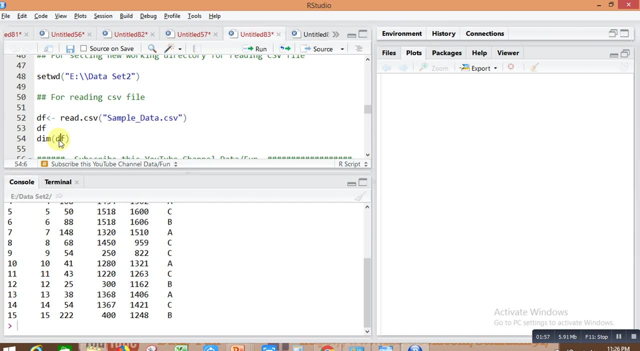 the type. so very simple and understandable data, and so so we will check the dimension of data by this command: dim df. there are 15 rows and 5 columns. so if you guys not familiar with the situation of outlier, i am showing one situation of outlier by plotting a box plot. you can also check the outlier in your variable by plotting a. 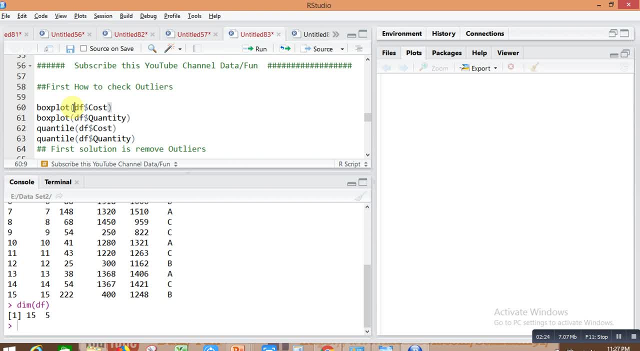 box plot. i am plotting a box plot for cost variable by this command. Box plot in bracket df and cost variable after the dollar sign. you can see here one value of cost column is so far from the rest of the values. so this is the outlier situation. similarly we can check the outlier in quantity column: same. 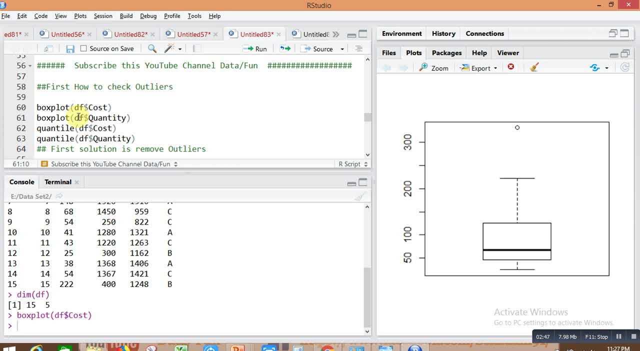 command box: dot df, dollar sign quantity. so you can see here all three values are given. so while this item- in case you are, alan, after this team, іc突um KM 아주 wale, if you see as time clicking two times in value, value will beОnt exactly. 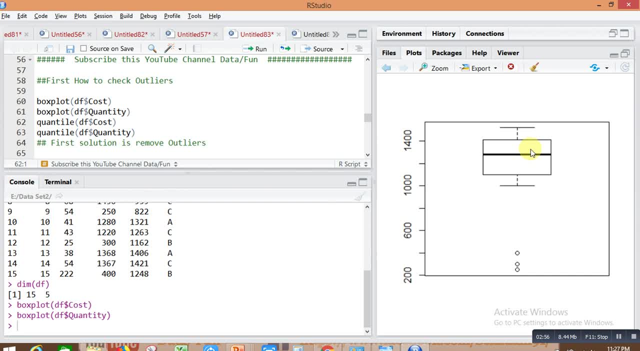 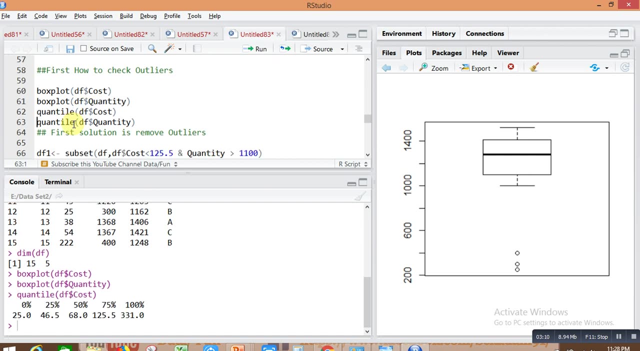 values of quantity are so far from the rest of the values of quantity. so this is also the outlier situation by. second option for checking the outlier: by calculating quantiles. you can see the outliers, see here. the last outlier, last quantile, is so far from the rest. 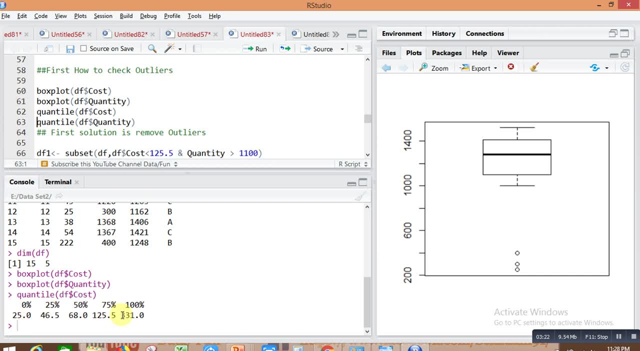 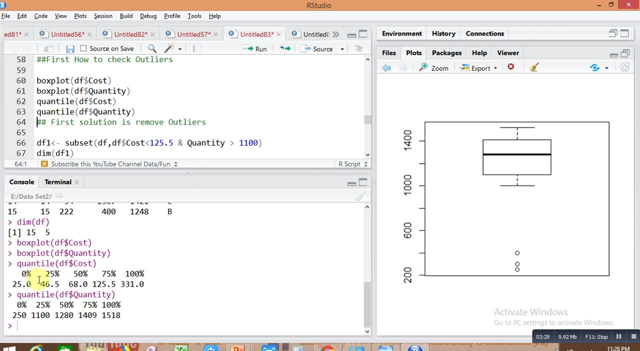 of the quantiles. so this is the outlier situation. second, we will calculate quantiles for quantity column as well. you can see all the quantiles are greater than 1100, but one quantile is less than and so far from the 1100. so this is outlier situation and for dealing this. 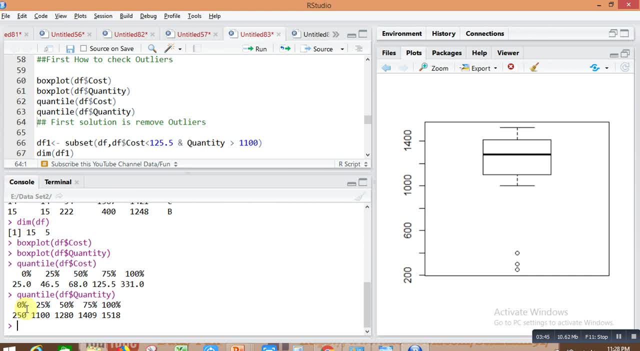 type of situation. first solution is remove these values directly in your data set. so this is first solution, and second solution is replace these values- outlier values- by suitable value. so first we will see: remove the all values- sorry, not all, only outlier values- in your data set. by subsetting you can remove the outlier values in your data set. i am removing. 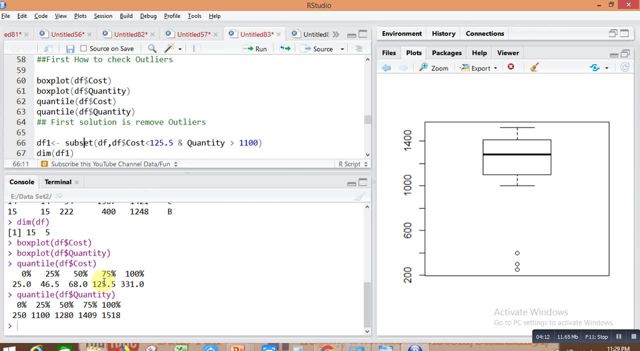 less than greater than 125.5 values- okay, from cost column and less than 1100 values in quantity column. so you can see here greater than 120 point, 120 point, 25 point, for you values are outlier and here is 1100 and less values are out there. so I am reviewing this: less than 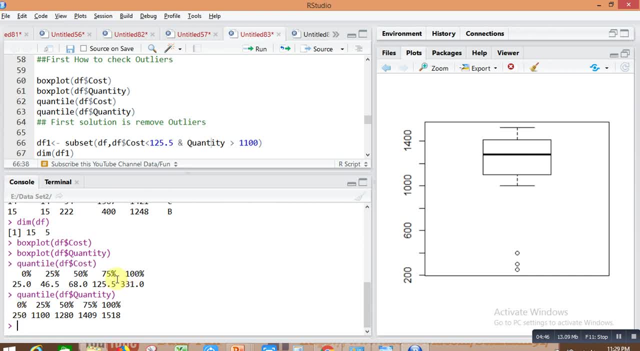 1100 values and greater than 120 for 25 point for you values. by this subset command you can do. I am giving new data frame, regenerating one new data frame, df1 subset our main data frame df, and if cost value is greater than sorry, only. 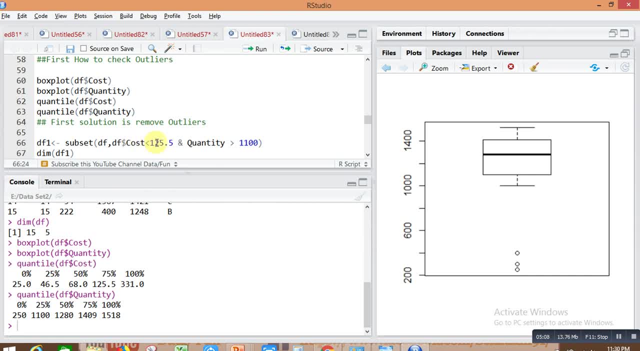 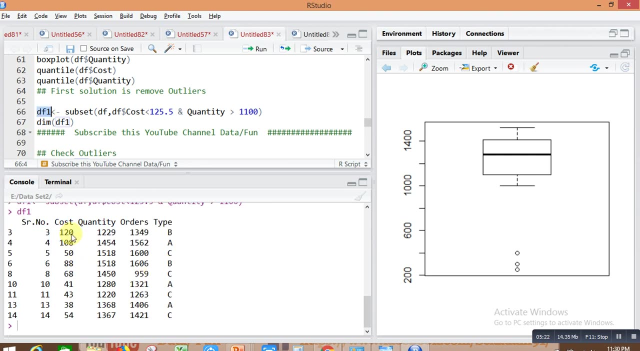 the cost values are less than the 125 point for you, and quantities are greater than or less than 125 point for you, and quantities are greater than or less than only 1100. so this is my new data frame name, df1, so you can see here all the 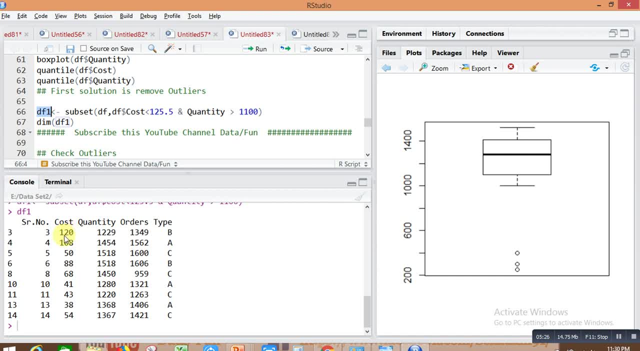 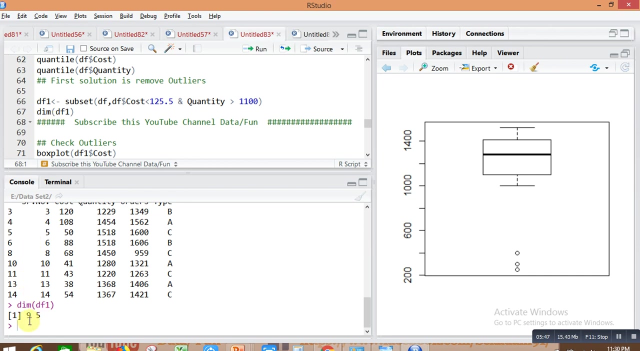 values above 125 are removed, and here all values greater than 1100 are removed, so this data becomes homogeneous. because of removing outliers, you can check the dimension dimensions also reduced: 9 rows and 5 columns. in our main data frame there are 15 rows and 5 columns, here is 9 rows and because of we. 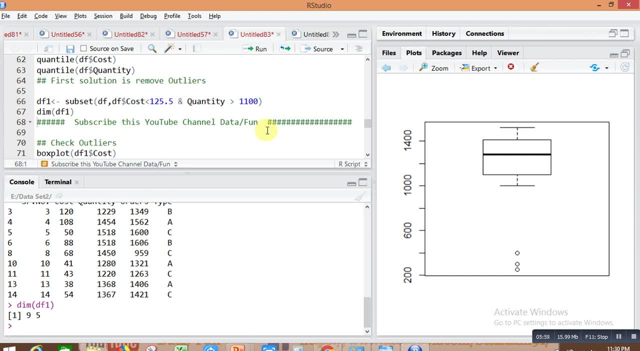 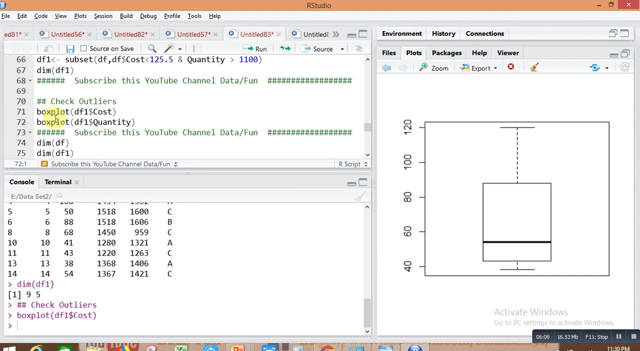 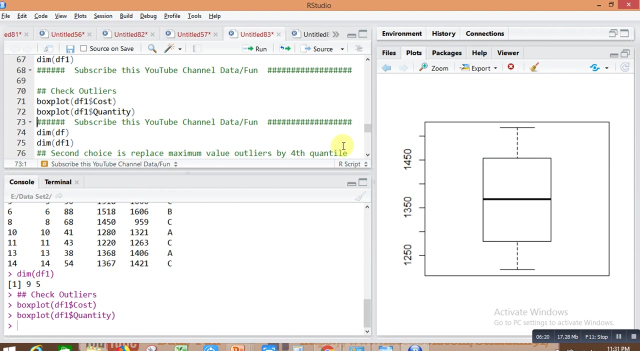 write here. condition: you can check the outlier for new data frame. just check any outlier in updated. there is no any outlier situation here because we remove these outliers similarly for lamb or there are no any outlier. this is first solution, directly remove outlier in your data frames. but this solution is not. 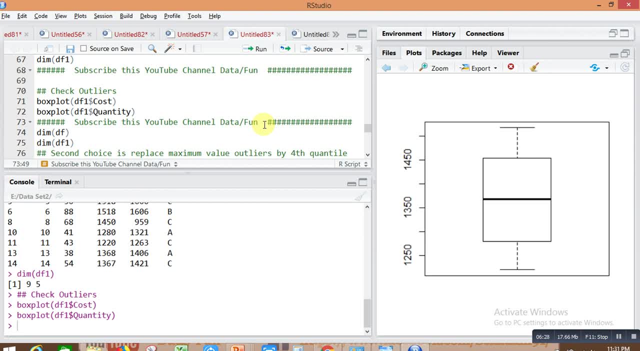 every time suitable, because these solutions directly reduce our information and that's why it's not a very suitable for the every time. so second solution is to replace maximum value. This depends on your ontology load position définition. ok, это прид должен быть из конт. 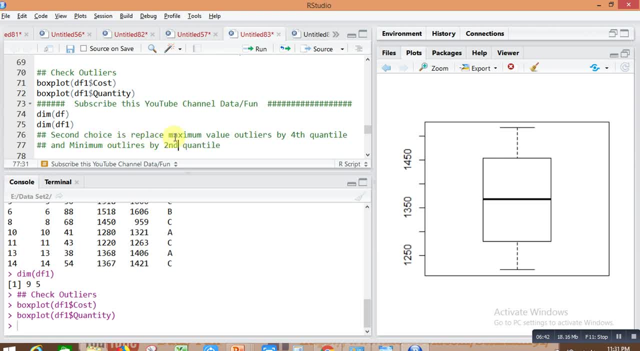 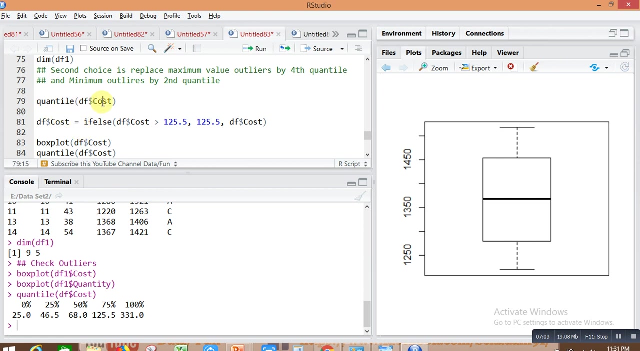 доع 90下 т Santo grinds ゲ're a you outlier by fourth quantile and minimum outlier values by second quantile. so let's see. first we will see for the cost variable. I am calculating quantiles for cost variable. this command quantiles DF, dollars and cost. so you can see here above 125 there are outliers. 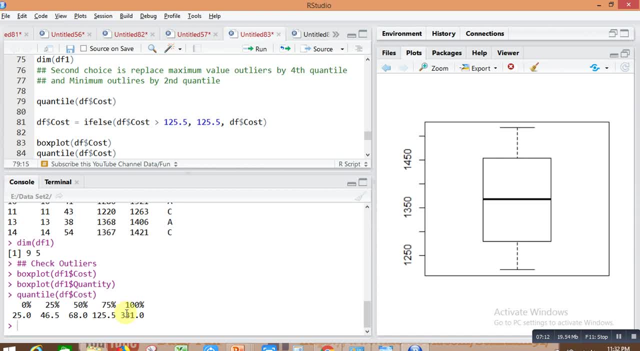 so I will replace all the above 125 values by 100, by 25. let's see by this: command DF dollars and cost. if else, condition DF dollars and cost. if values are greater than 125.5, replace the value 125.5. if not, then write this values as it is. 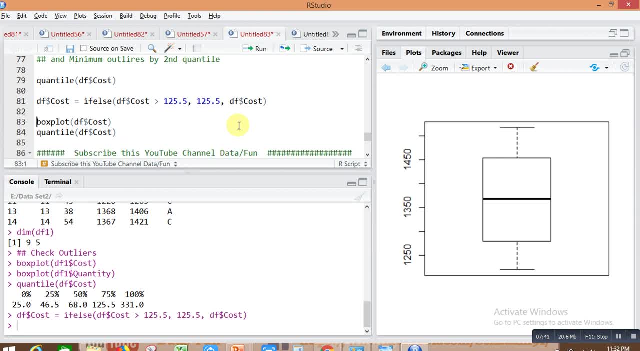 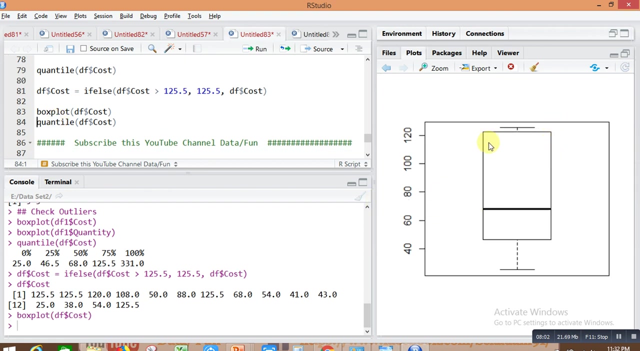 you see the cost column. you can see here all the greater than 125 values are replaced by 120.5. just plot the box for new, updated column. you can see. all the outliers are converted into the homogeneous data same. I am calculating quantiles for the cost variable and minimum.